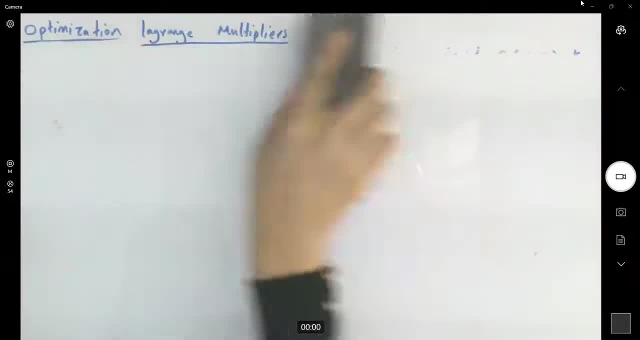 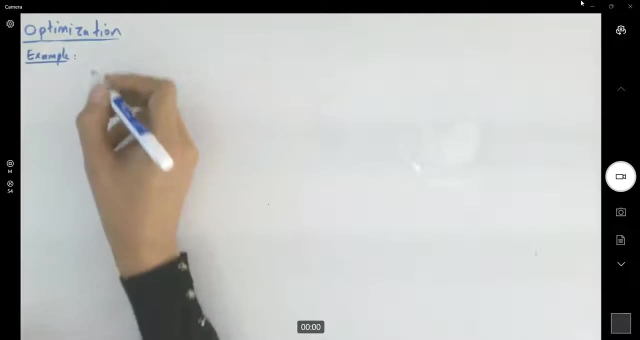 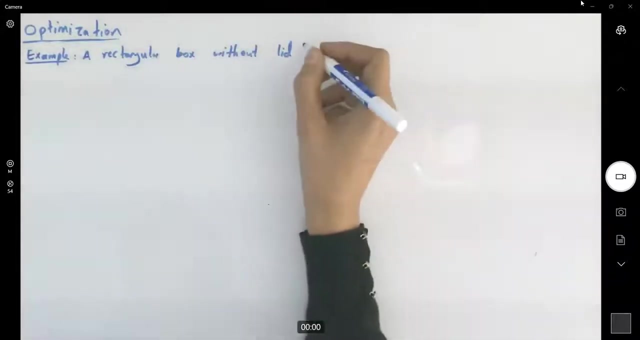 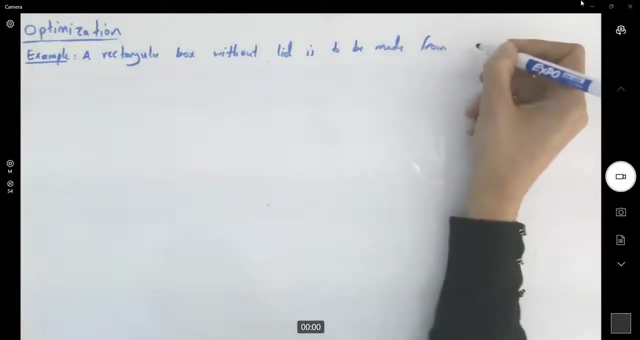 erase this because i need space. at the same time, i'm going to write down the steps in applying Lagrange multipliers. so in this example we have the following scenario: a rectangular box without a lid is to be made from 12 square meter of cardboard. okay, so far, so good. so far we have some pieces of information. find the maximum. 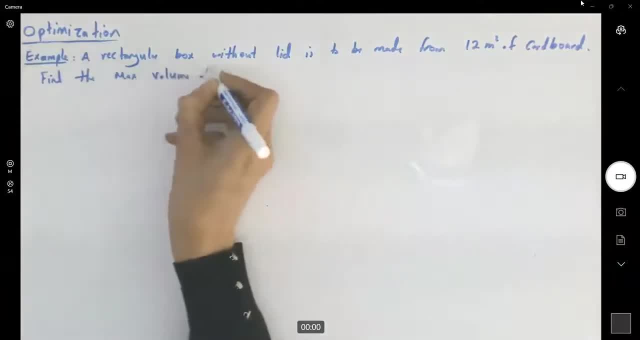 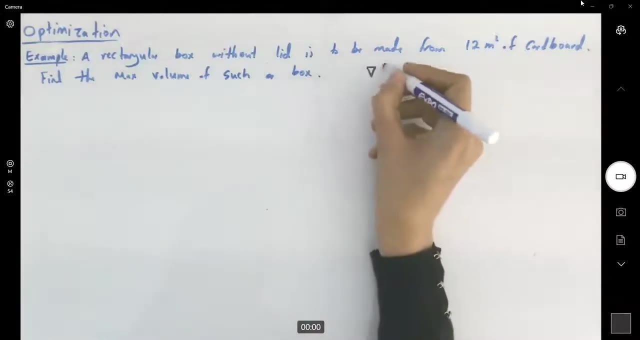 volume of such a box. okay, very good. what is our goal? our goal is to identify what f is. take its gradient and set it equals to lambda, the gradient of the constraint, which is function g. function g has always some constraints, or something like that. so it's our goal to know what f equals. the rest of the order of the box. 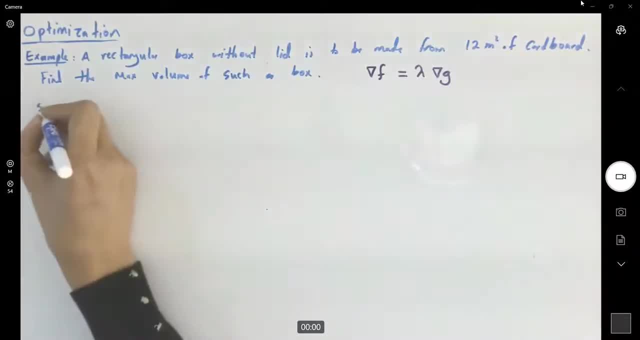 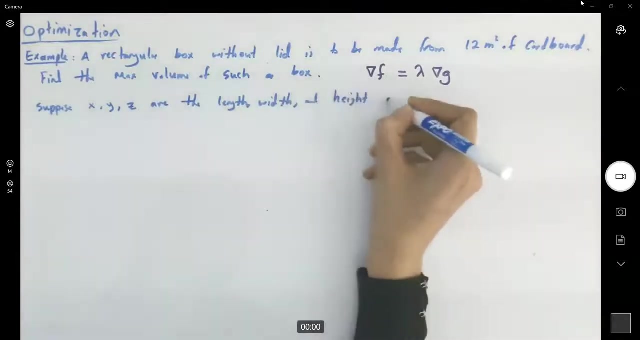 so we protected the x and the y from their stories from the order of the top to the bottom of the box. so i'm going to start by collecting the volume of a box. okay, i'm going to write down those terms And the height of the box. 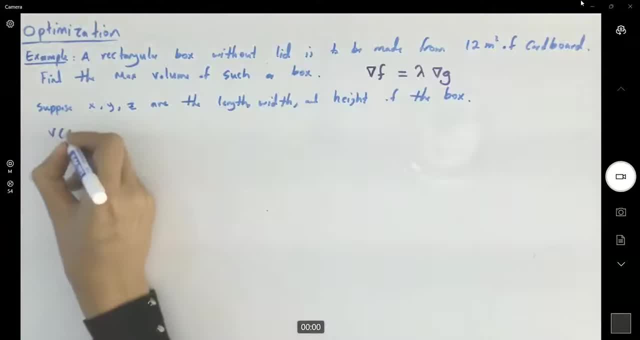 So what's the volume formula? The volume is x times y times z. So we try to maximize this function. This is your f, this is function f. Now what about the constraint? What about g? Our function g Of x, y and z is equal to 12.. 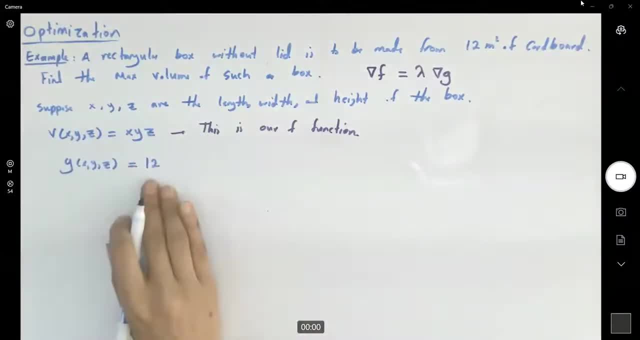 But how do I formulate this function? I have my k, but what's the relation between x, y and z? Remember that we're trying to create a box with a lid to be made from a 12 square meter cardboard. Your function g, the constraint, can be written as 2xz plus 2yz plus xy equals to 12.. 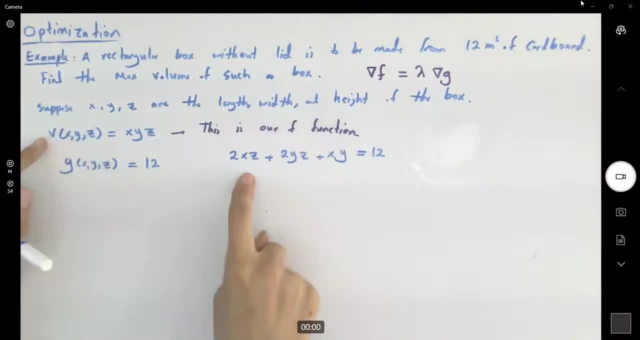 I have my volume, I have the constraint. Now I'm going to apply the Lagrange multipliers method. So, gradient of my volume, which is gradient of the volume, The volume which is the partial derivative with respect to x, yz. 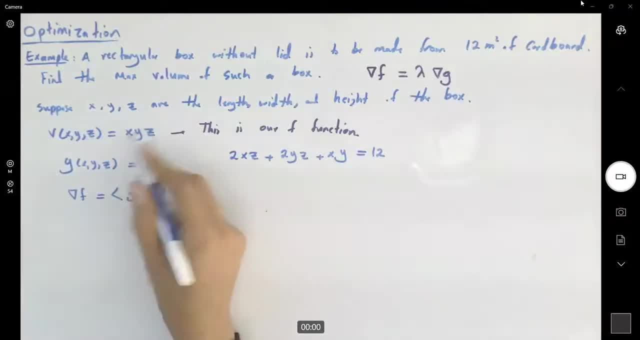 The partial derivative with respect to y- xz. The partial derivative with respect to z- xy Is equal to lambda, the gradient of my constraint. With respect to x, I have 2z plus y. With respect to y, I have 2z plus x. 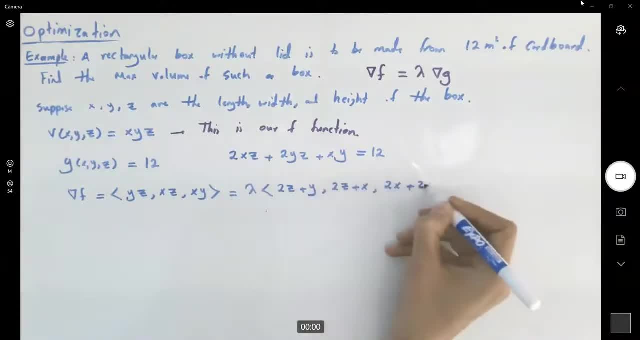 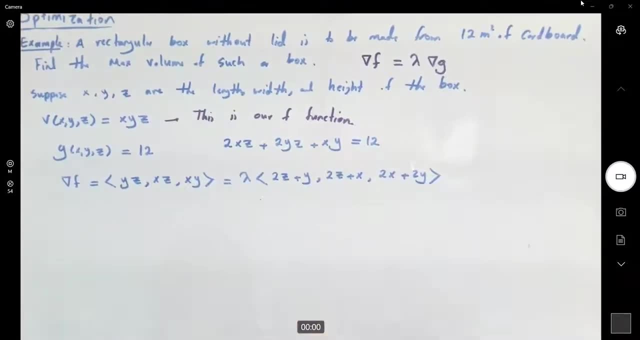 And with respect to z, I have 2z plus x. I have 2x plus 2y. I'm done with the calculus part. Now pure algebra. Okay, let us begin. We have yz equals to lambda times 2z plus y. 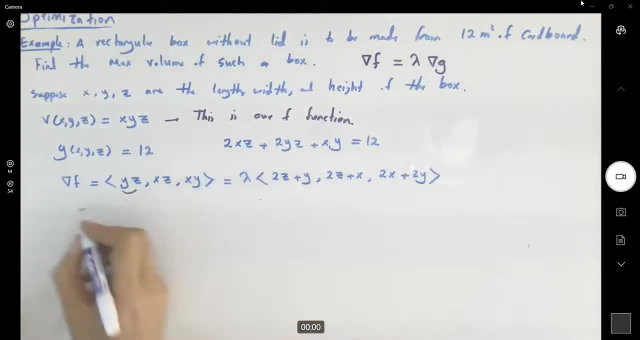 yz equals to lambda times 2z plus y. yz equals to lambda times 2z plus y. I have xz. I have xz, equals to lambda. Remember that you have to distribute your lambda into each component: Lambda parentheses: 2z plus x. 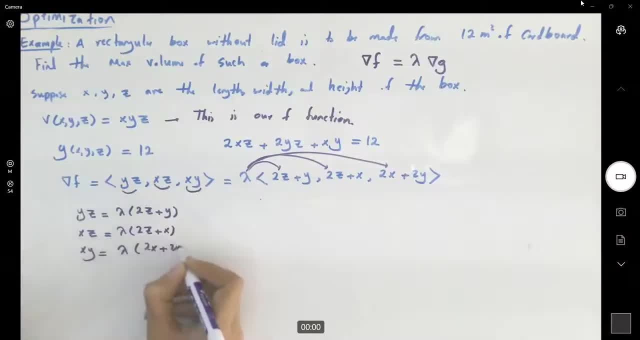 And you have xy equals to lambda function x plus 2y. Here we go. We also know that there is a relation between xy and yy. also know that there is a relation between xy and zy. and on the right hand side we have 12.. Now take a look: My yz is equal to lambda 2z plus. 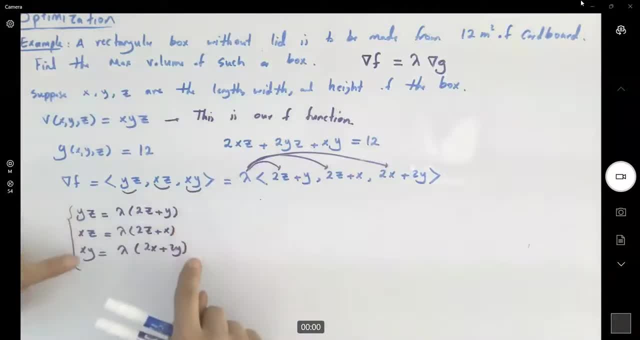 y. If I multiply each one of these equations by the missing variable, I'm creating the following system: I have x, yz equals to lambda parenthesis, 2, xz plus xy, Multiplying the second equation by y. So here I have x? yz. 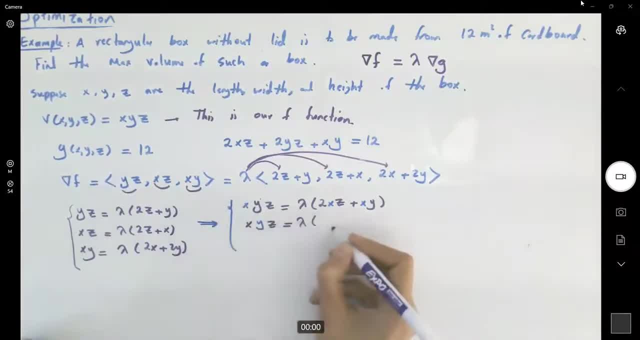 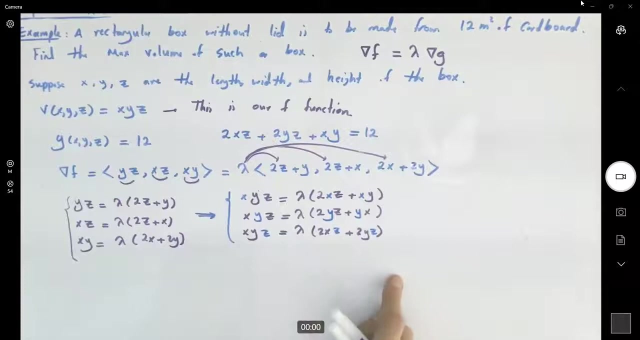 which is equal to- lambda- parenthesis- 2 yz plus yx for xy. And finally, multiplying the last equation by z, xy, z equals to lambda 2 xz plus 2 yz. There we go. So what is the next step here? for me, All of these are equal to each other. 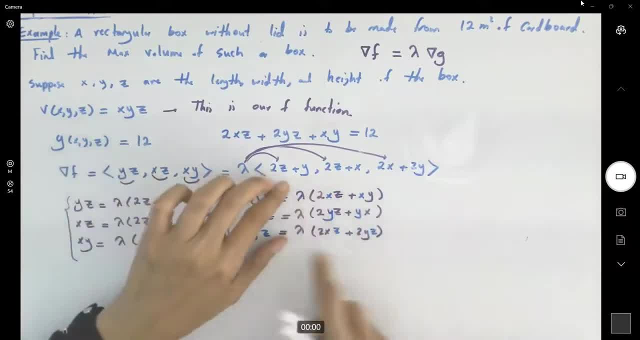 xy z equals to xy z equals to xy z. It means I can set these equations equal to each other Two by two, Right? So let me set these two equations equal to each other. let us call it equation one, equation two, equation three: set one equals to two. if you set one equals to two, you can cancel out lambda and. 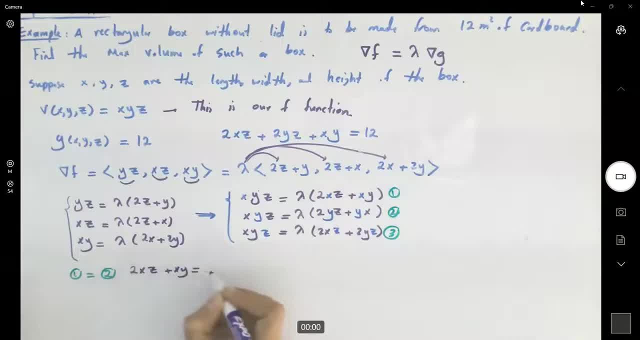 you get two xz plus xy equals to two yz plus xy. okay, so, as you can see, you can cancel out xy and you get two xz equals to two yz or x equals to y. so far, so good. x is equal to y. i'm going to use this equation one more time to get the missing elements very good now. for example: 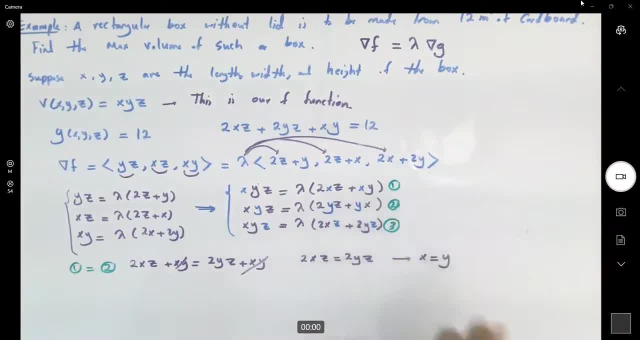 you can set one and three equal to each other. you can set two and three equal to each other. let us set two and three equal to each other. if two is equal to three, then what do we get? we get lambda and lambda, they cancel out. we get two. 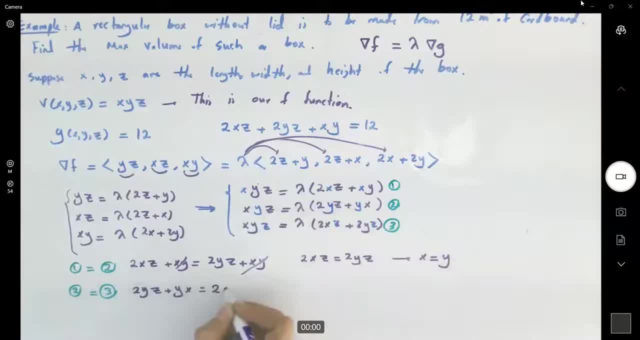 yz plus yx equals to two xz plus two yz. so two yz, two yz. and here you have. let me see. in this case you get y x equals to 2xz, or you get your y equals to 2z, so my x is equal to y, my y equals to 2z. and then let's see what else I can do. 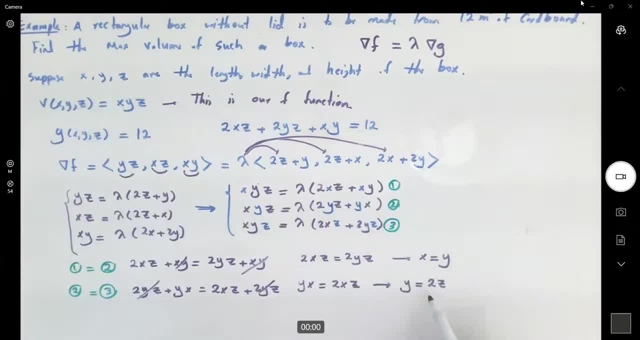 and x is equal to two yz plus yz plus two yz plus two yz plus two yz. prices zwischen y, y, y, x and y x, z. all right, so i'm going to sum all these, sum all these down to y and z and this is it, and i'm 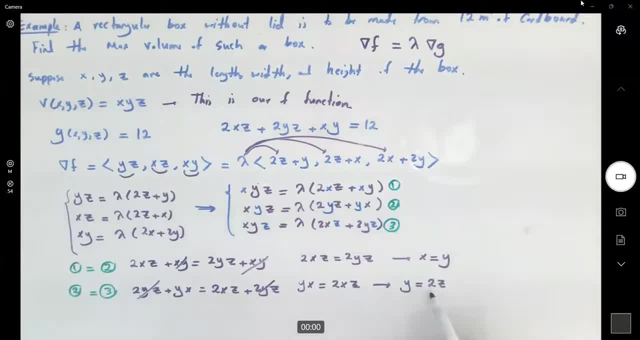 gonna be fitting all this in into my equation one by one. break it up a second. so let me recognize this. i'm going to do this term fighting term against being equal to seven and n is equal to j and j is equal to xx. so let me add: and under 전 j and j, if you type n equals to Kakadu. 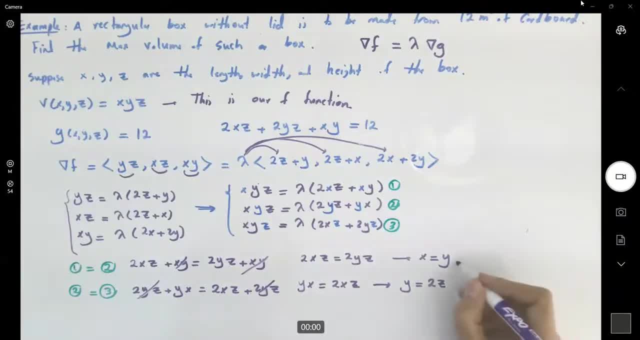 this, this term fighting term against you. that's a very important factor because people aren't automatically equal to 2z. So so far I have all the information that I need. I'm going to use the constraint and find my z value. Use the constraint. It says I have 2xz, 2, 2z times z plus 2, 2zz. 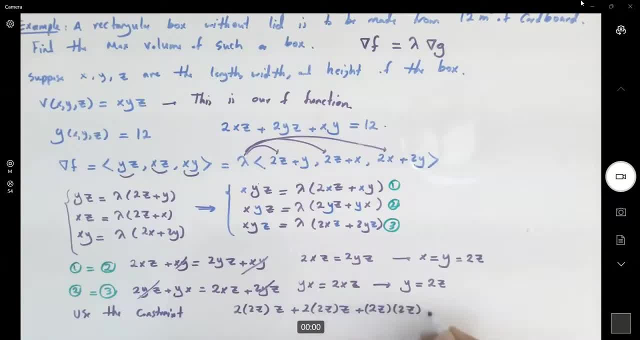 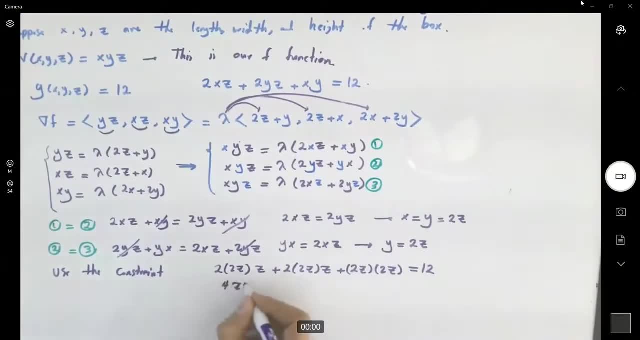 plus 2z times 2z equals to 12.. Okay, very good, I have 4z squared plus 4z squared plus 4z squared equals to 12.. 3z squared is equal to 3.. So z, as the length is equal to 1.. 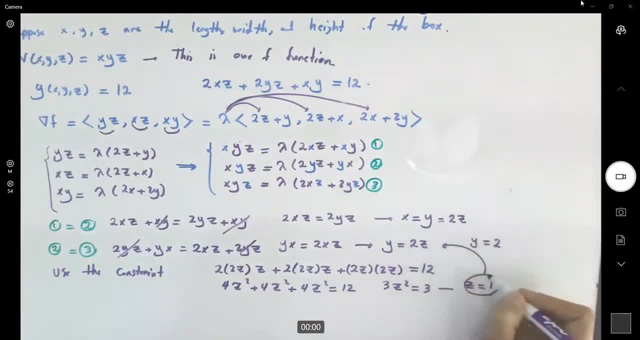 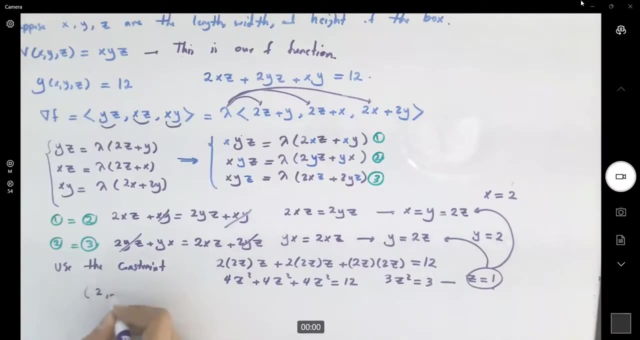 When z is equal to 1, y is 2,, x is 2.. Very good, So I have found my x, y and z. 2,, 2, and 1 is the point or the measurement where we get the maximum. 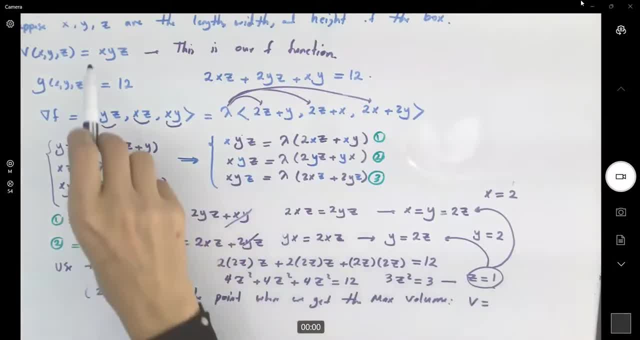 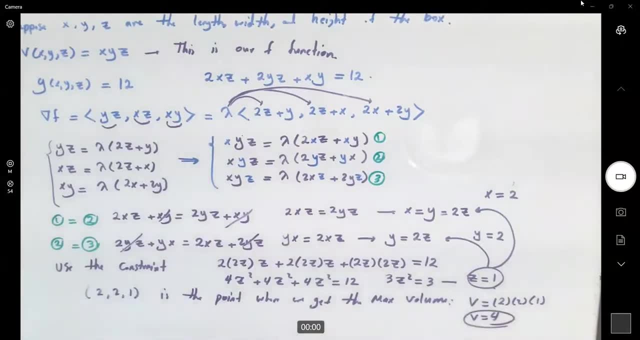 volume. The volume is x, y, z, 2 times 2 times 1, or the volume is 4.. The constraint is the surface area for your box, Surface area. So if you have a box with the base x, y, x, y and the height z, the area of this box, the surface area for this box, is: 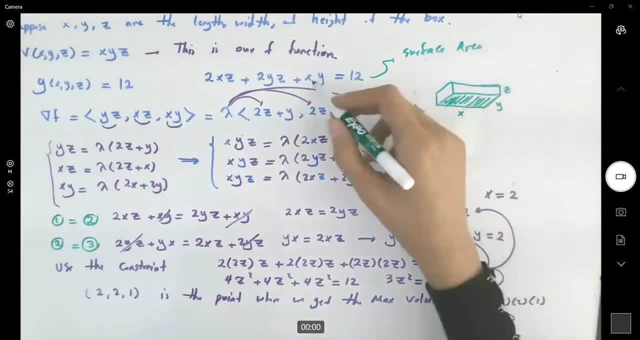 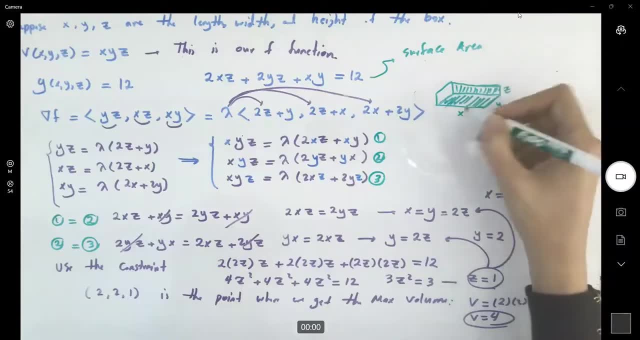 the area below, which is the base x, y. Then you have two parallel sides, which is your xz plus xz hat. So you have, and also you have. So you have 2 peroầu giys, which is 2 perov fra global. Then you have a little short place. 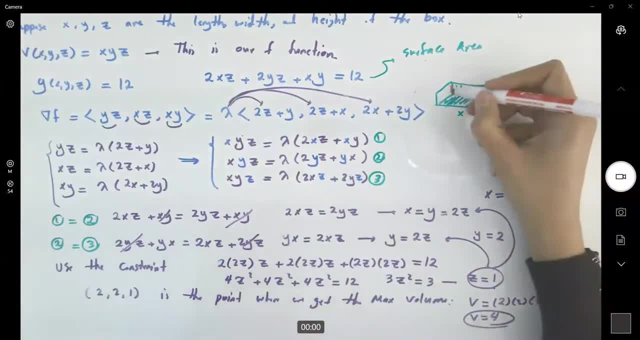 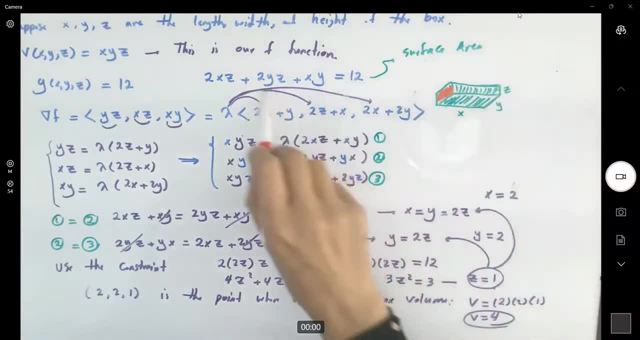 you have these two sides which are parallel to each other. It's going to be YZ, one YZ here, one YZ on the other side of the box, so you get two YZ.